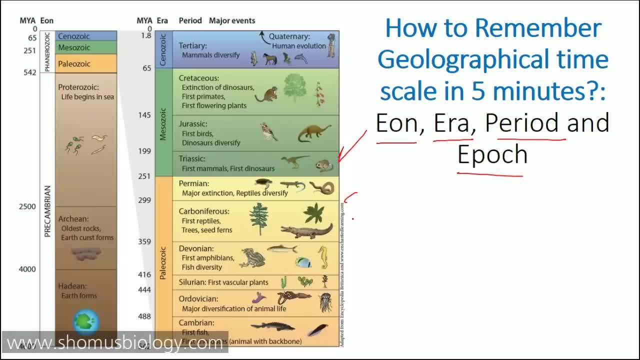 From scratch, you will be able to draw this whole table on your own without looking at anything else after watching the video. So I dare you to watch the video. 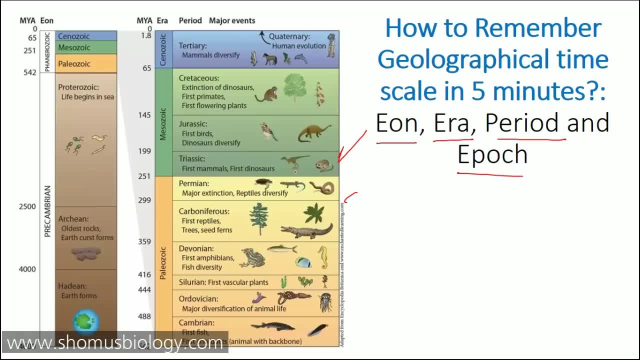 So you need to know three things to answer this particular table. The things are few pale buttons, a camel and egg in a plate. These are the three things that you need to know, right? So how exactly if you peel buttons the way a camel can sit, and eggs on your plate help you remember the geographical timescale. If you're wondering 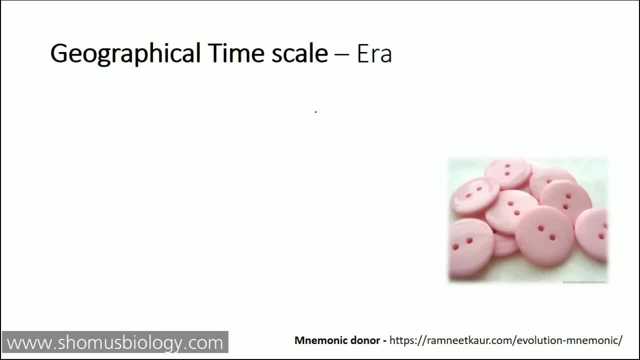 about that, let's look at here. The first thing that you need to find out is era how to know and how to get era. To get era, there is a sentence that you need to remember and that sentence is press the pill button to message the center. Yes, that's how easy it is. 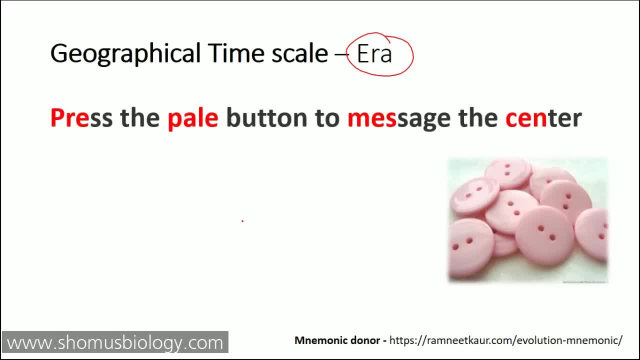 Press the pill button to message the center. So it starts with the steps like press PR ego with 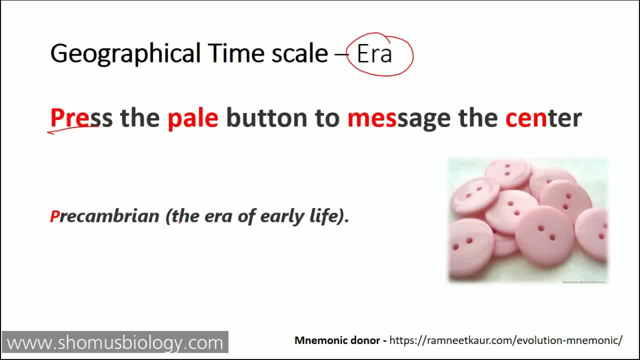 ES em Cristiano because they steps people around the area. Because as we all know, we've come home. So the first step is to make, yes, we're going to be able to do this now. 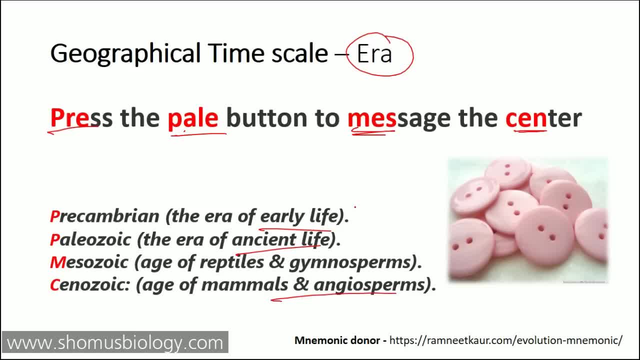 The second step is the the third- dome which fits something this chart. So the third step is timeитьi erba messing between birth and expiration. And we are. Again, The third step is time itroycambrian era. The era is the first era in the early life span. Then pale. The era of ancient life. 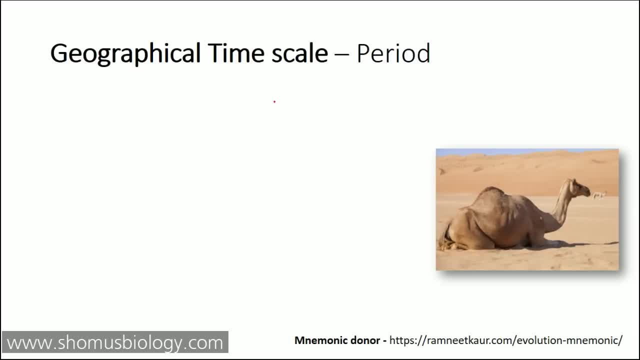 to remember geographical time scale period to remember geographical time scale period goes with another sentence camels often sit down carefully perhaps 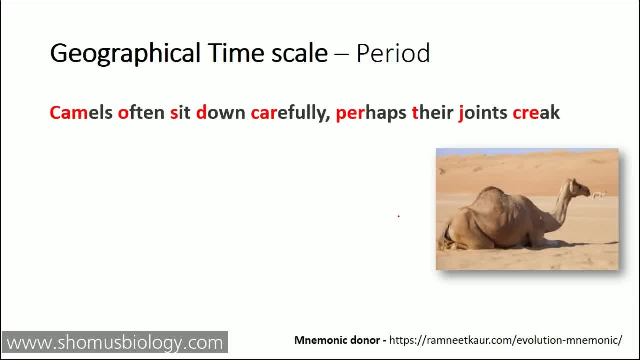 their joints creak well yeah they are big fella maybe their joints creak 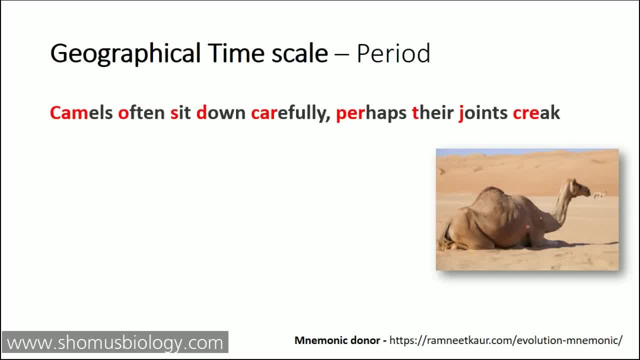 that's why they sit down often and their sitting position is kind of weird as you can see so let's begin with the first one of the period cam so Cambrian in the 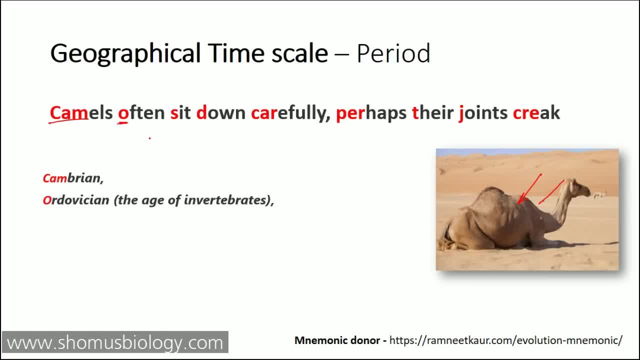 first one or starts with oh the second one or do vectorj then the third one is s silurian then the fourth one was D Devonian right remember one thing for each of this like Odor vision is the age of invertebrates and devonian is age of fishes and abundance of tree of ferns then see a are carboniferous the age of amphibians the first seed plants appeared in this part then thứ vào P-E-R, Permian, origin of conifers, then with T, Triassic, then with J, Jurassic, the age of reptiles, dominance of gymnosperms, and C-R-E at the end, Cretaceous, the dominance of flowering plants and mammals like us. 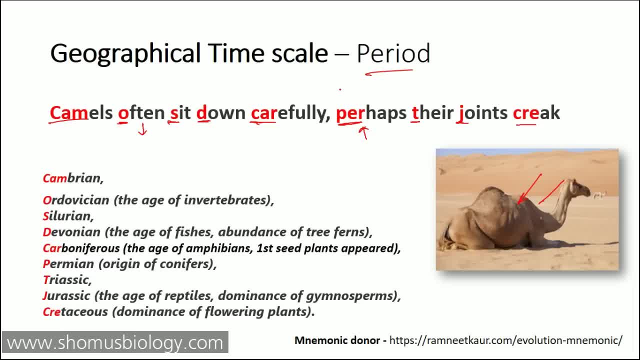 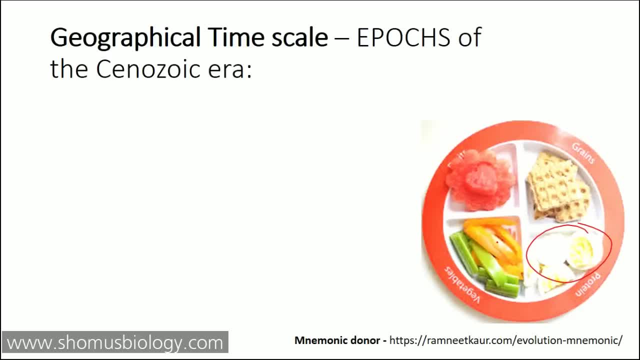 Now, as you know the period, the last thing that we want to know is the epoch. And to understand epoch, you need the third picture that is eggs in your breakfast plate. Give me some scrambled eggs. And actually, you're asking the scrambled eggs to your wife. So, you see simply, put eggs on my plates, please honey. That's what you're saying. Put eggs on my plate, please honey. 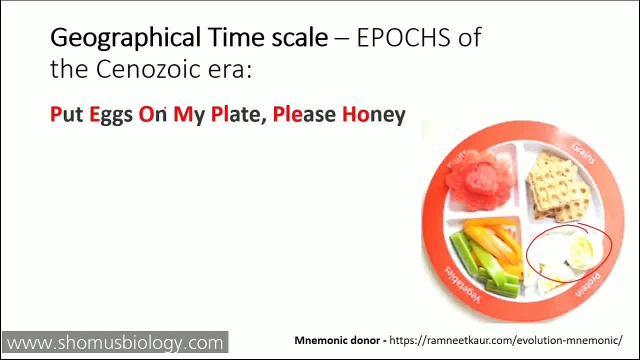 If you know this sentence, you can get the idea of the epoch of Cenozoic Era because this is the epoch of Cenozoic Era. 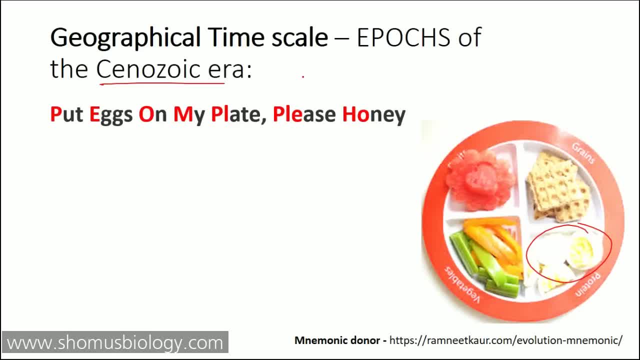 We are currently and you need to know the details and different divisions and epochs of this era. So, you go with this Cenozoic Era starts with P, Paleocene, then with E, Eocene, then with O, Oligocene, then with M, Miocene, then with P-L, Pleocene, and then with P-L-E, Pleistocene, and then with H-O, Holocene. 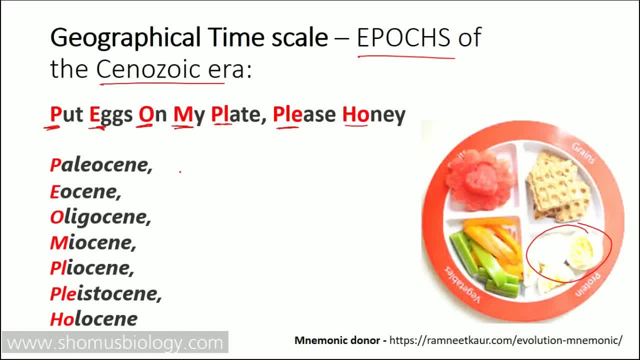 So, that's what you know, put eggs. On my plate, please honey. 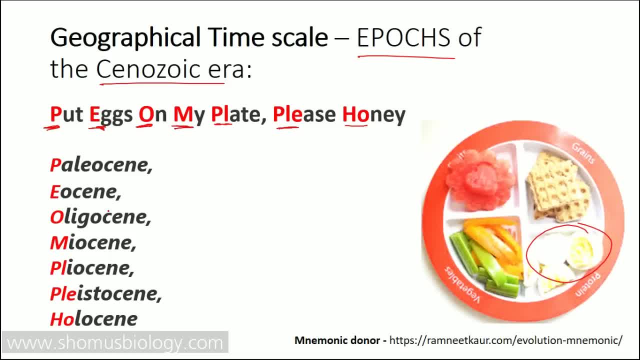 Starts with P-L-O-C-E-O-C-E, O-L-E-C-E-N-G, M-O-C-E-N-G, P-L-E-O-C-E-N-G, P-L-E-C-E-N-G, H-O-L-O-C-E-N-G. Just remembering the breakfast plate that you have. So, now you know if you remember pale buttons and how to press them. If you remember the way camel sits and bunch of eggs in your breakfast plate. 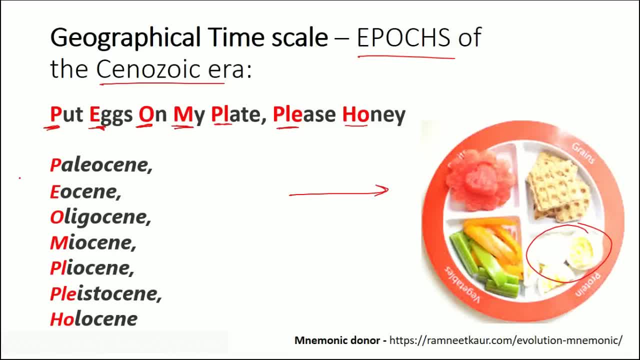 You need, you can easily find out the geographical time scale which was huge to understand.